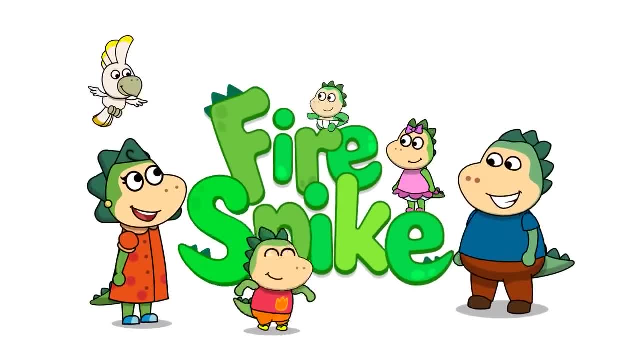 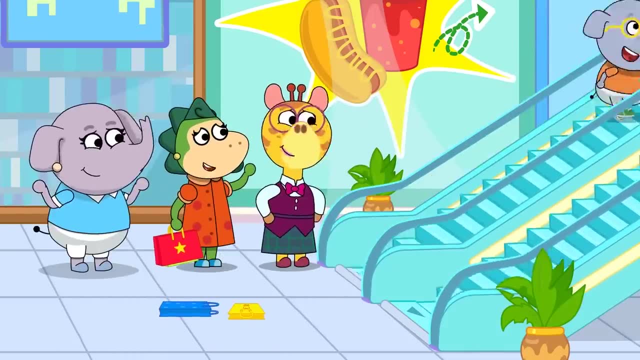 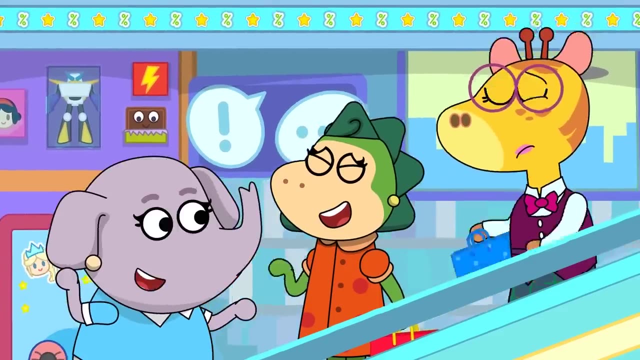 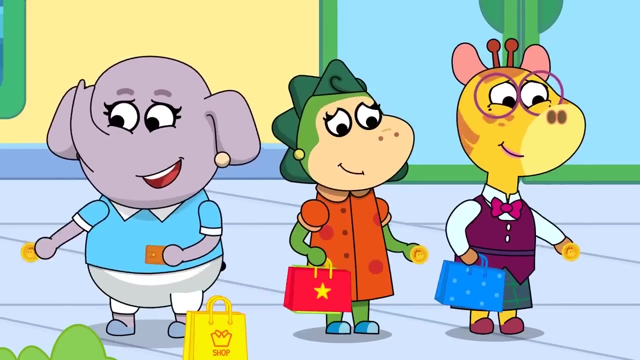 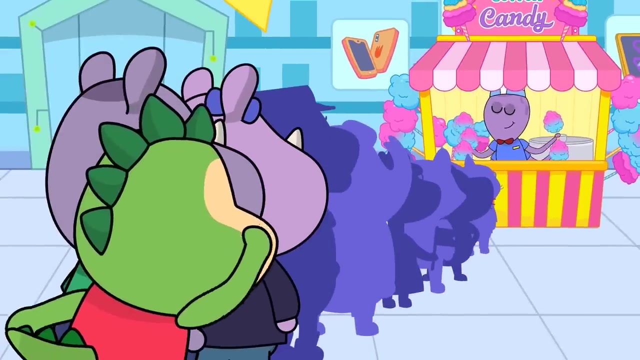 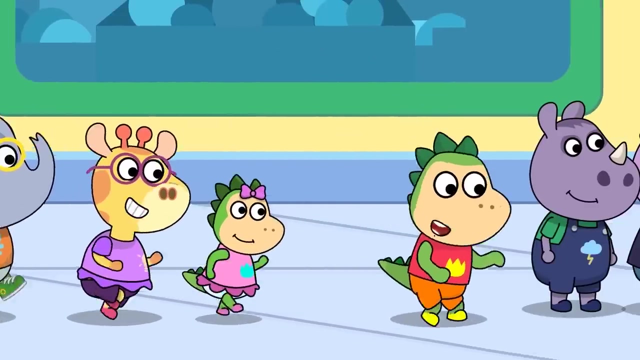 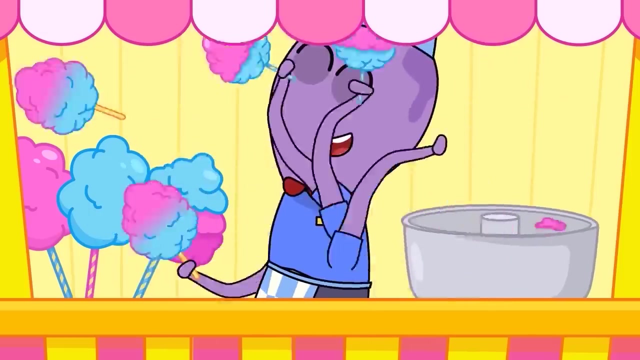 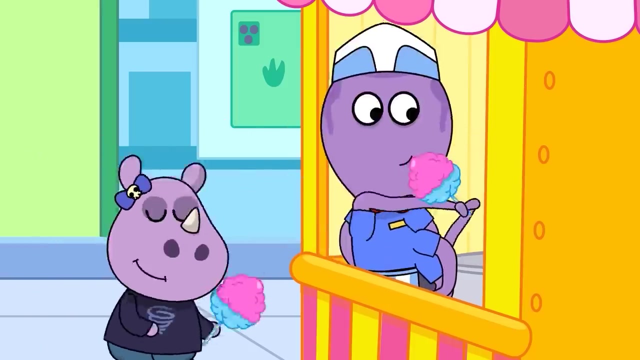 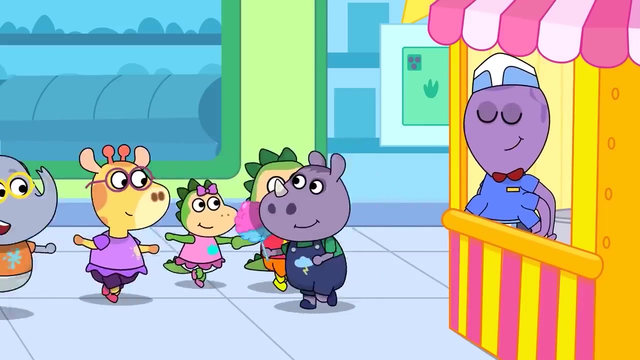 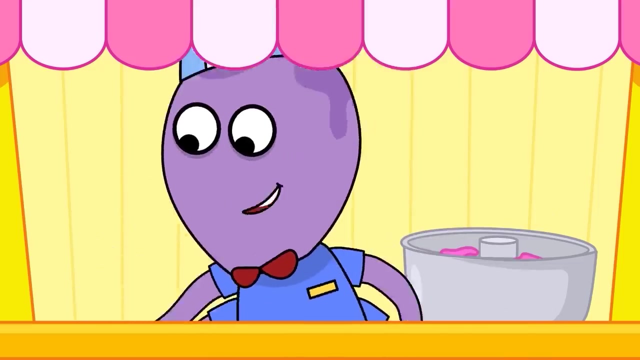 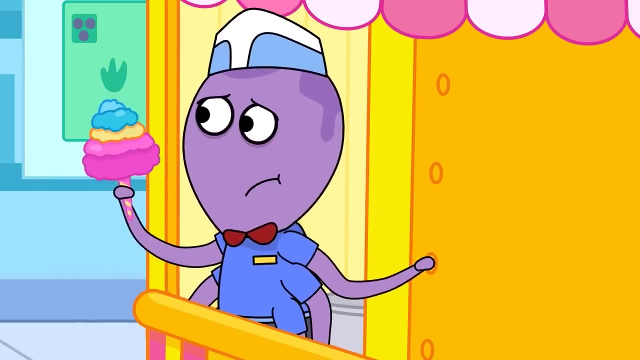 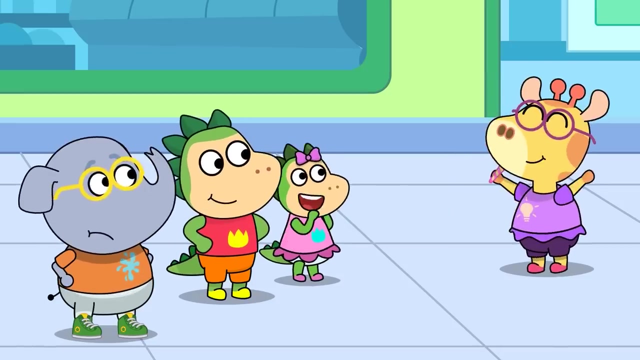 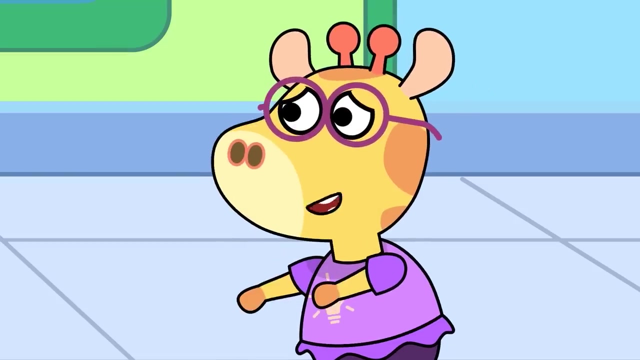 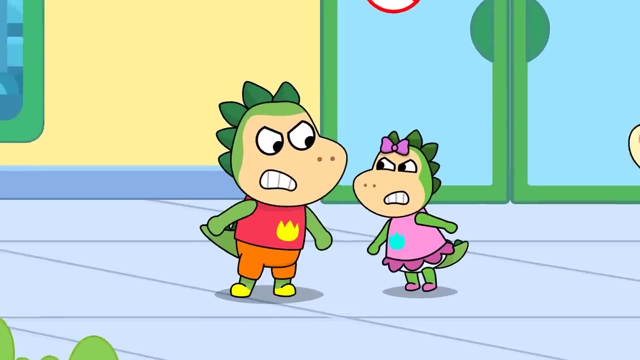 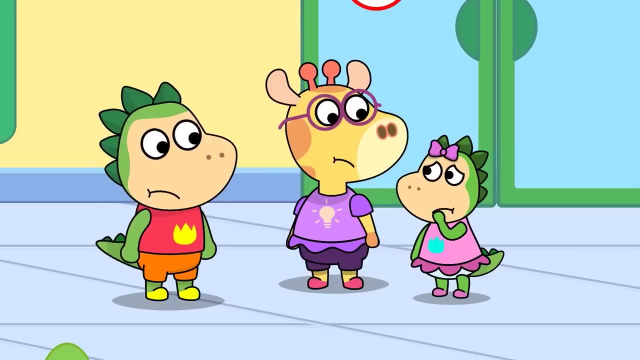 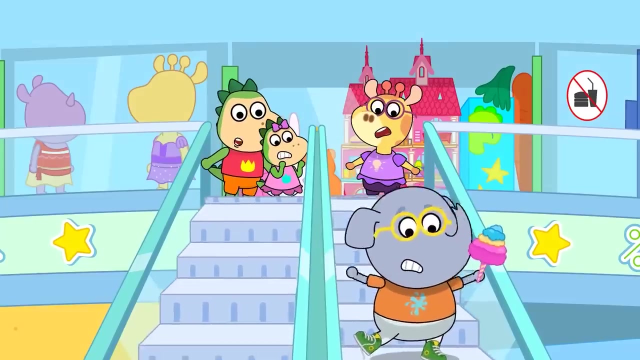 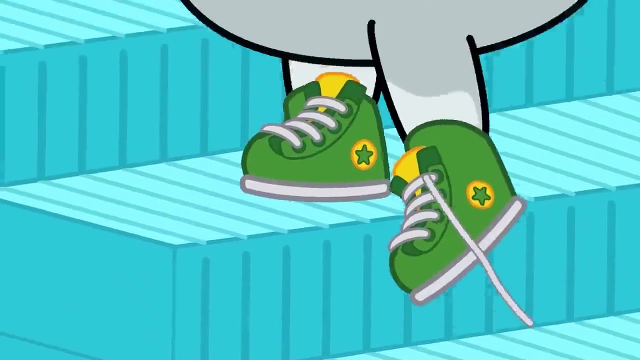 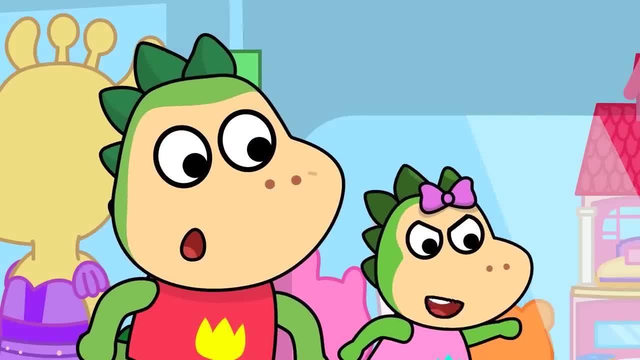 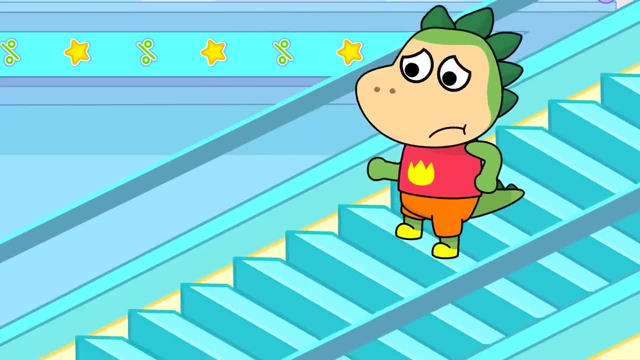 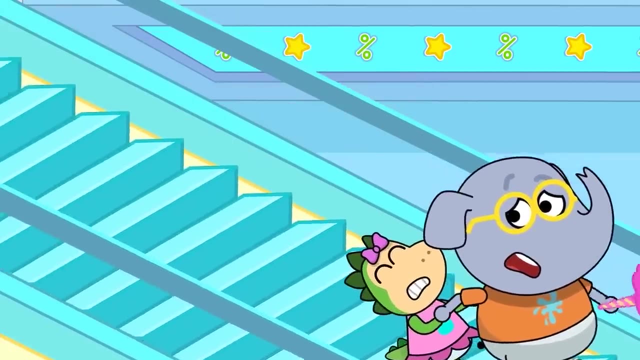 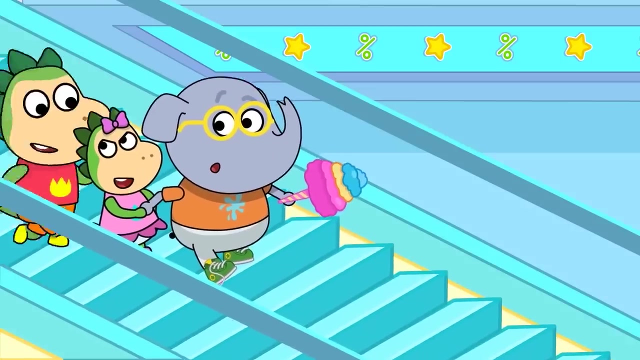 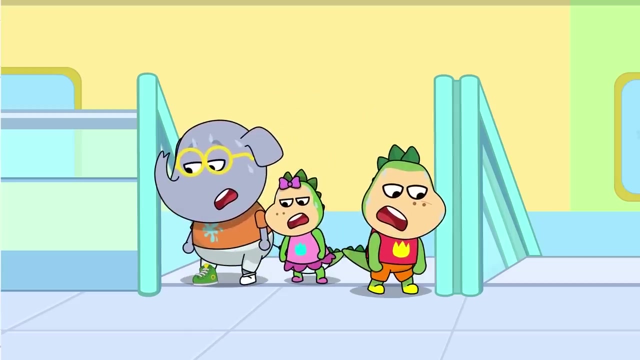 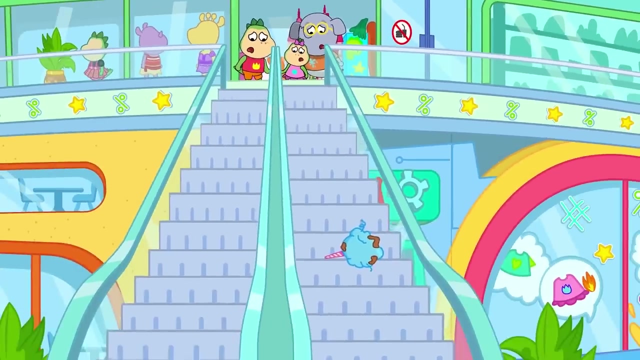 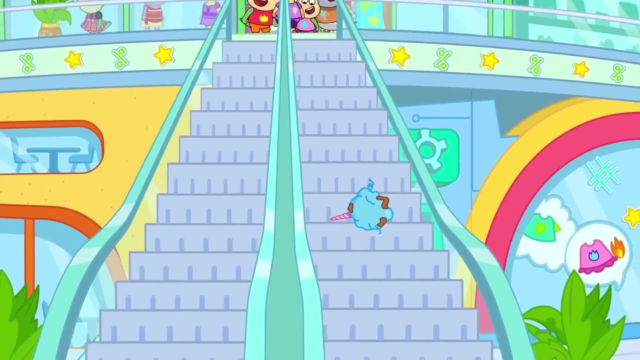 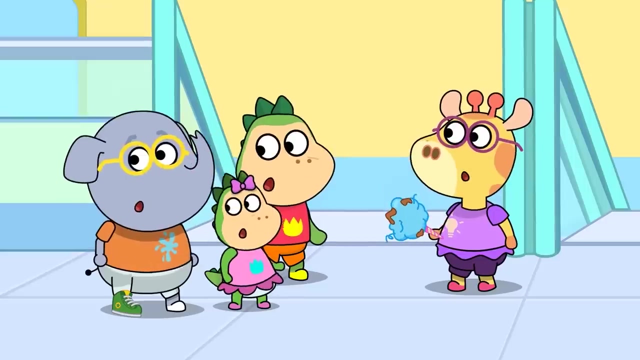 Please subscribe to our channel for more videos. Please add punctuation in the appropriate places. Please subscribe to our channel for more videos. Please add punctuation in the appropriate places. Oh no, Look, No, Yay, Aw, kids Hooray. 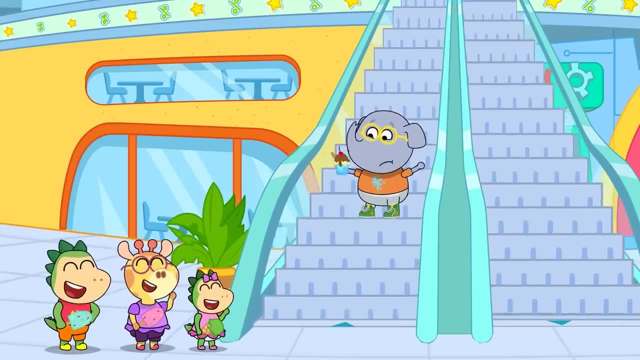 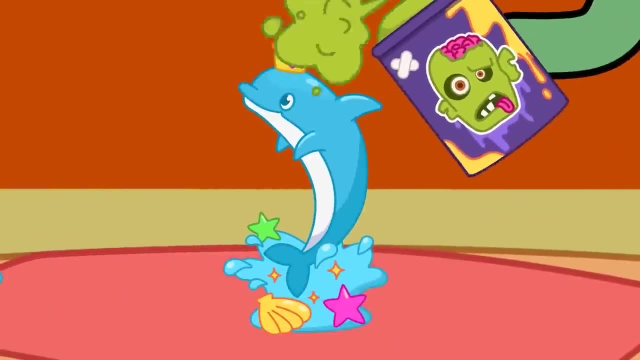 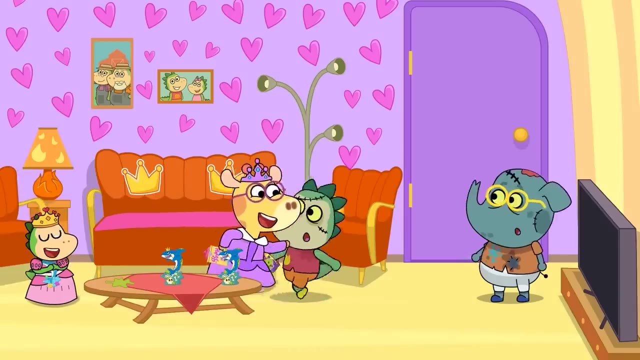 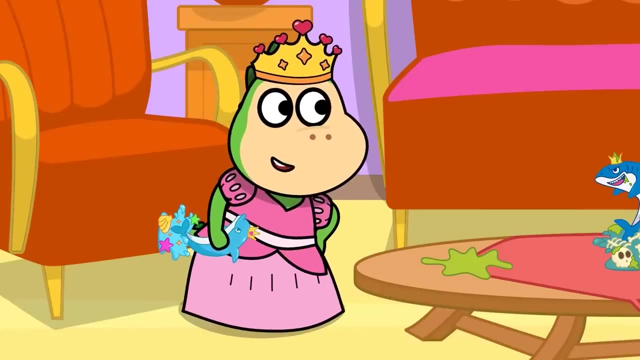 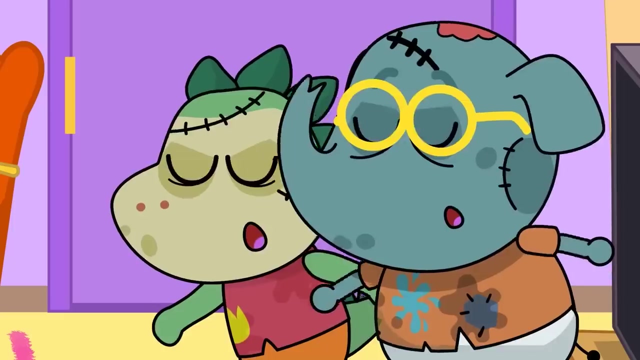 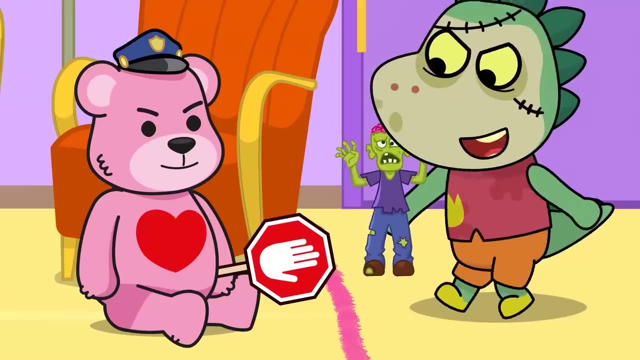 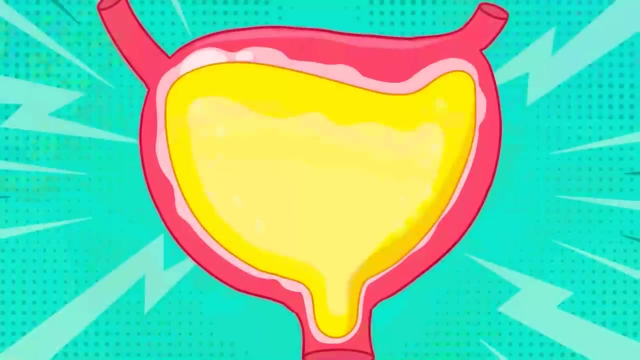 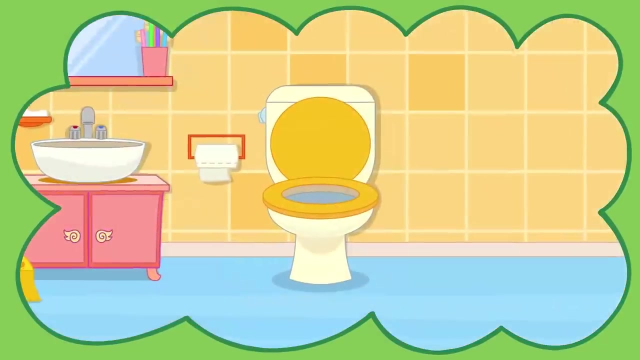 Huh, Help. Oh, Let's play fair. This is our half and that's your half. Only those in pink outfits are allowed to step in our kingdom. Huh, Challenge accepted, What? Hmm, Uh-oh, Hmm. 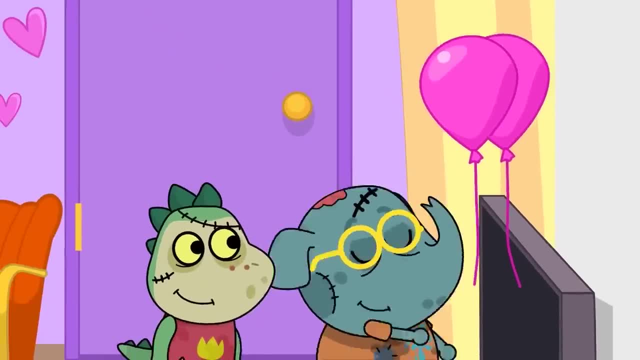 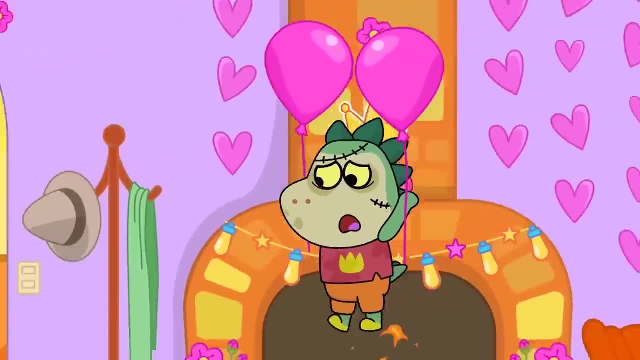 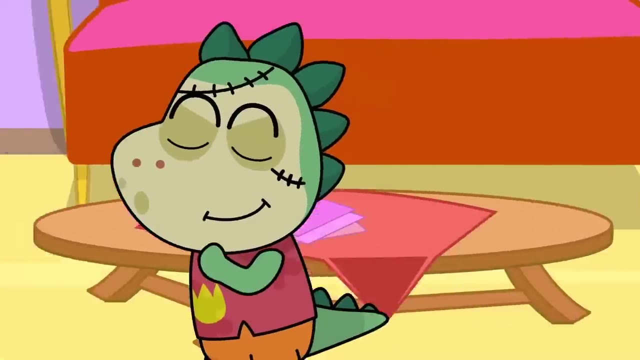 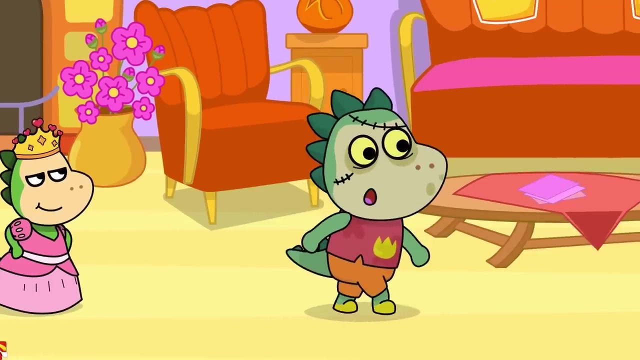 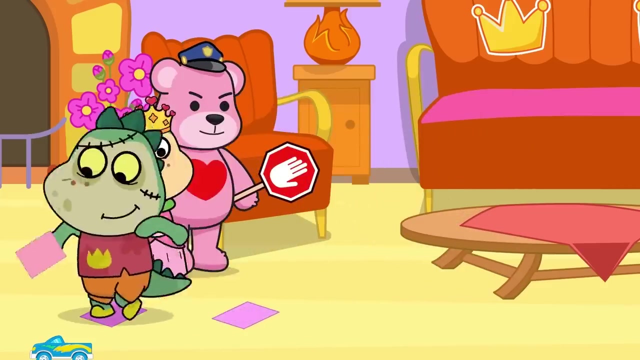 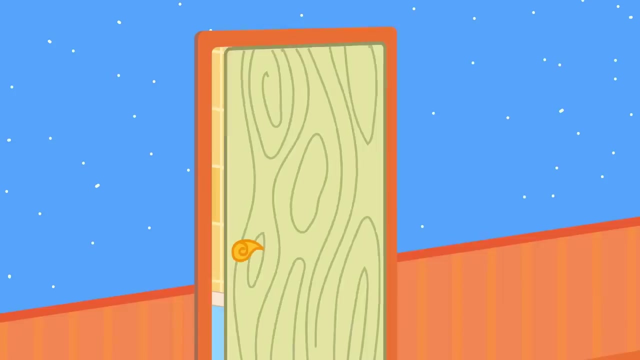 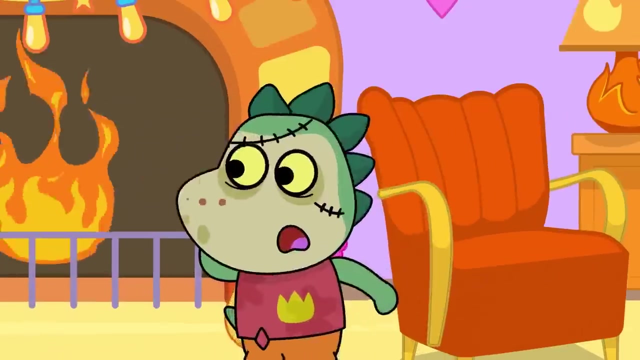 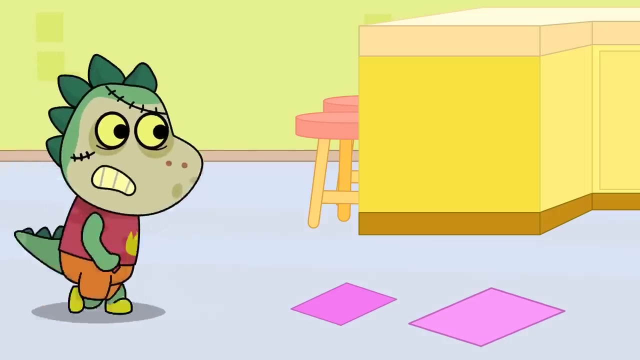 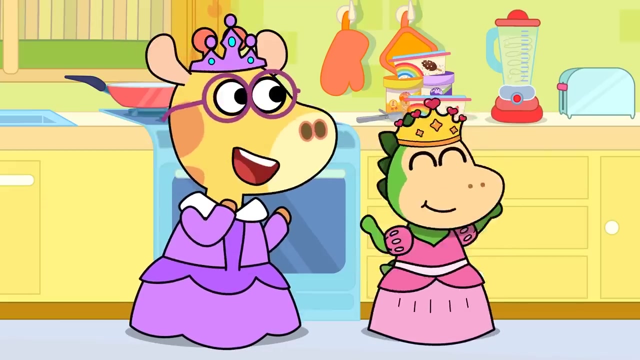 Uh-huh, Uh-huh, Uh-huh. No, no, the cars must be pink. What flavour would you, princesses, like to have in your milkshake Chocolate? And what about you, boys? Huh, But they're zombies. 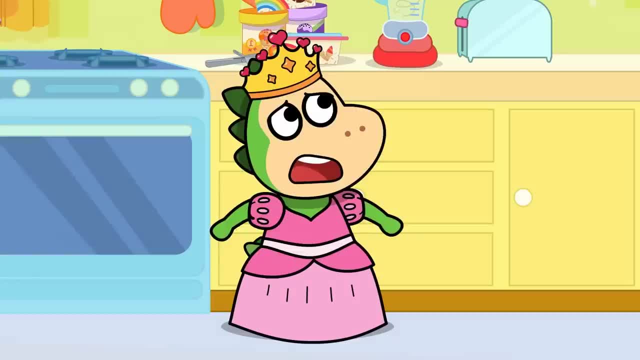 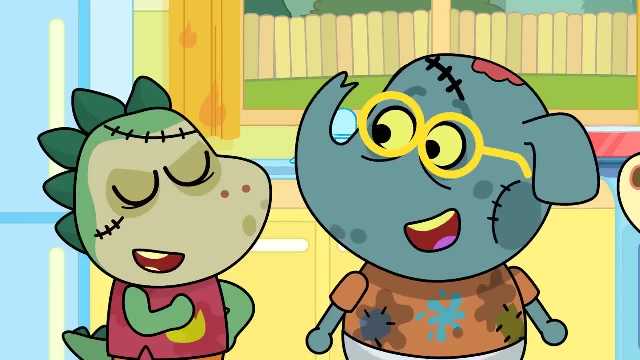 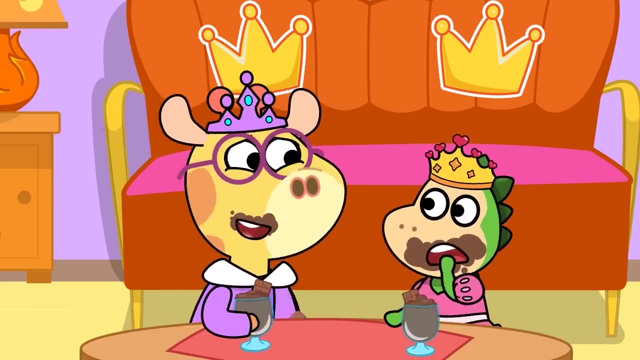 Really. Hmm, what flavour do zombies prefer? Oh, no, No, no, no. I like strawberry flavour And I'd love raspberry Sparkle. You're a princess, Sorry. I just like how Spike and Muggles look. 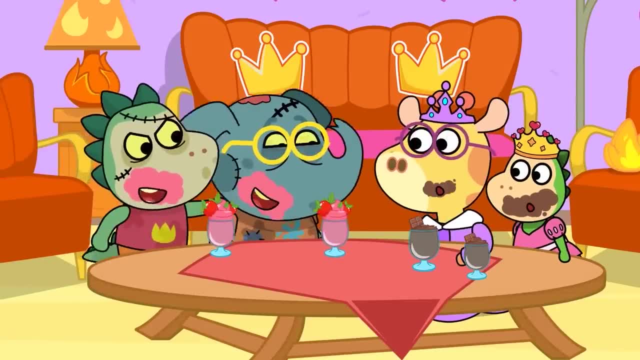 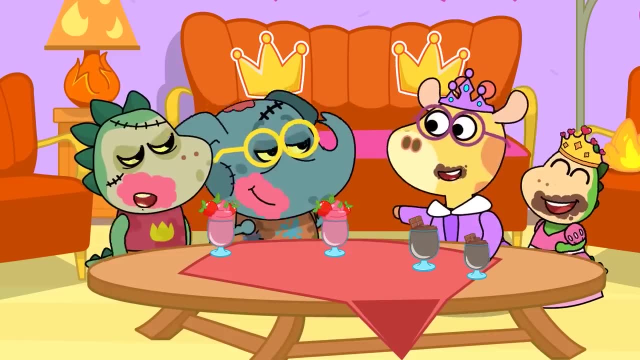 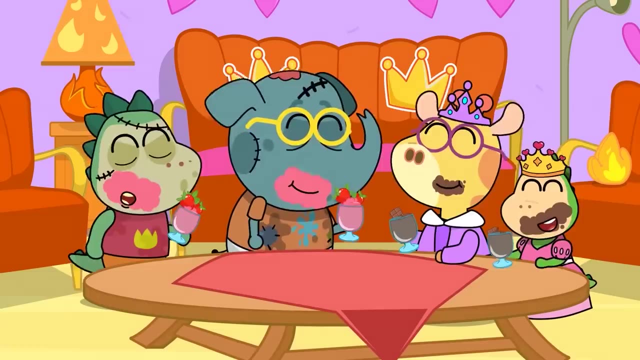 You're drinking pink drinks? We won't. Aha, Take a look at yourself, you. chocolate highness, Sparkle Your face And your face. You'd better look at yourself, boys. Huh, It's time for your shot. 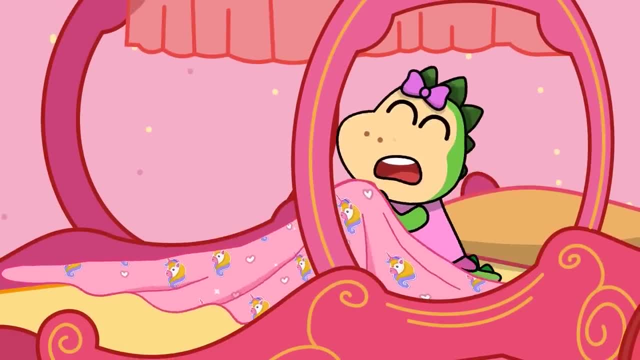 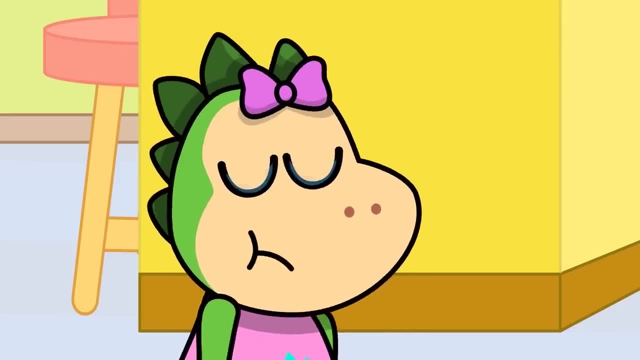 Huh, Barbie, What happened? Sparkle, Did you have a nightmare Come? It's all over now Have some pancakes, But eat fast. Today we go to get your shots. Who's next? Oh, no, Bowen, Oh. 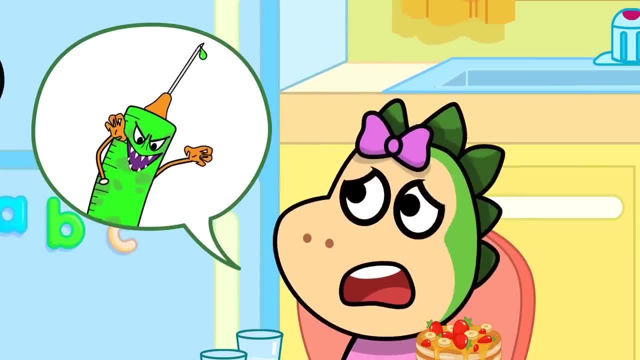 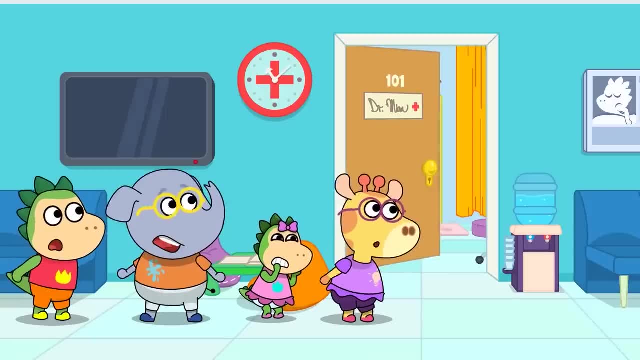 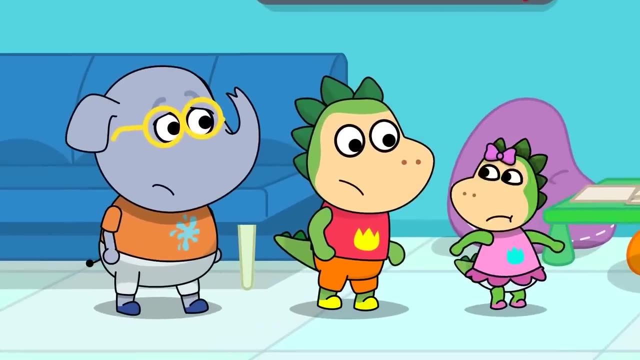 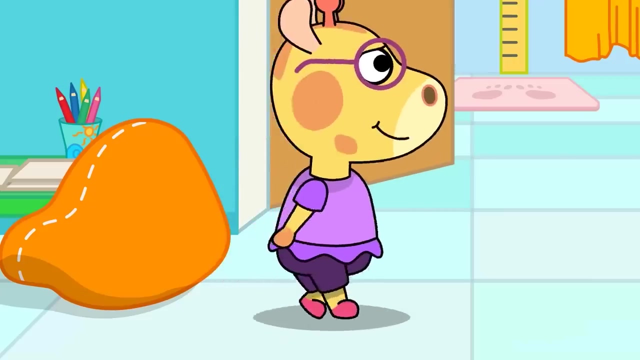 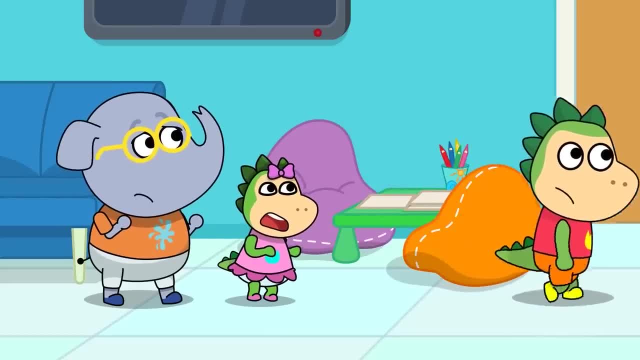 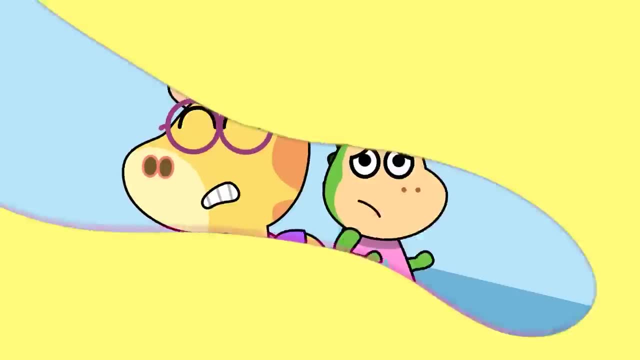 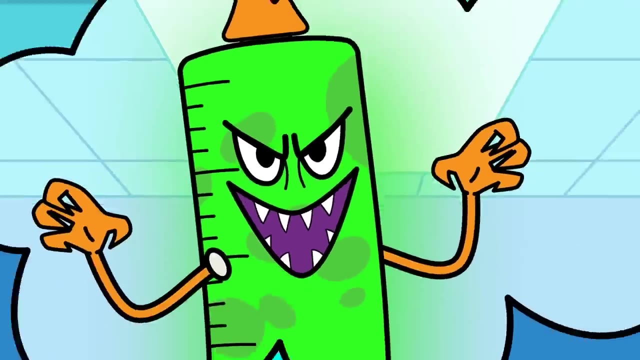 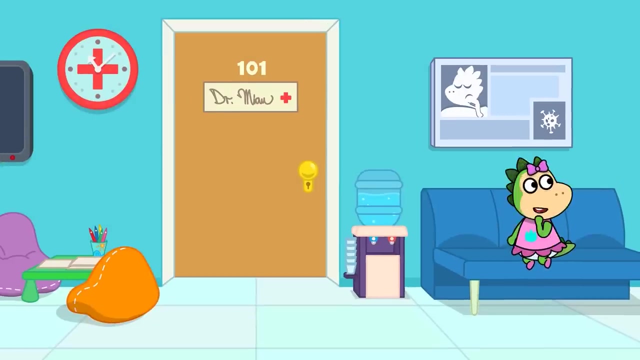 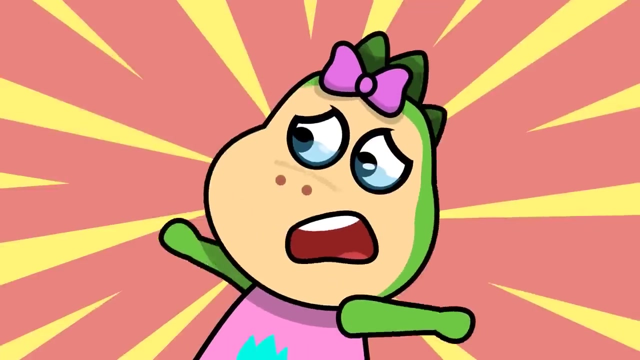 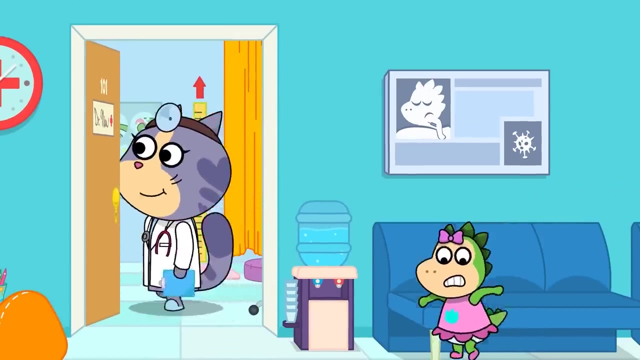 Next: Hmm, Uh, You go first. Uh, Uh, имер, Ah, Everybody run, Hiyah, Hiyah. Oh no, where's Muttles? Sparkle, Sparkle. You're next. Did it hurt? 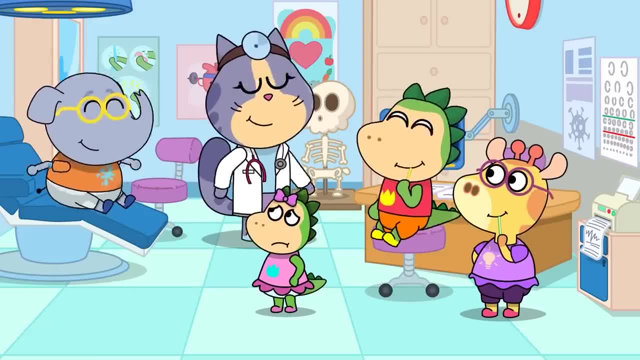 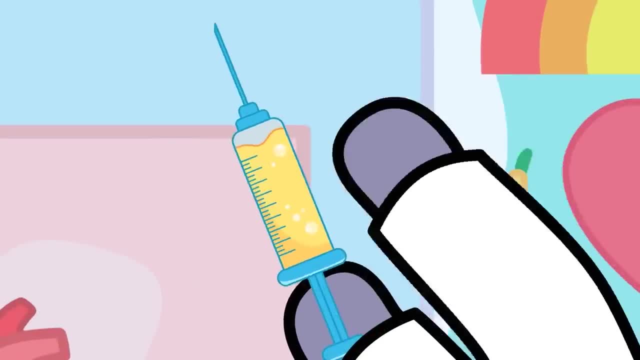 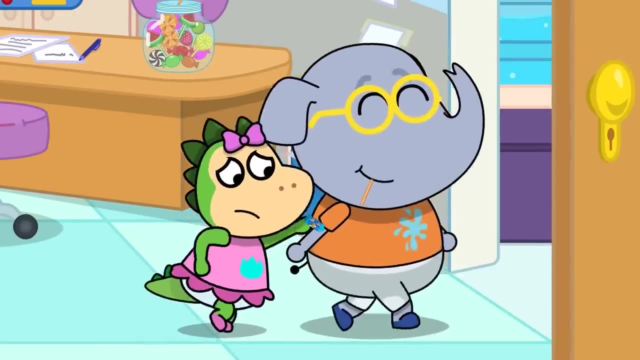 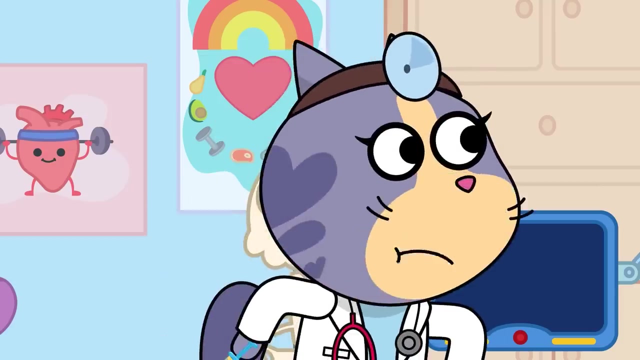 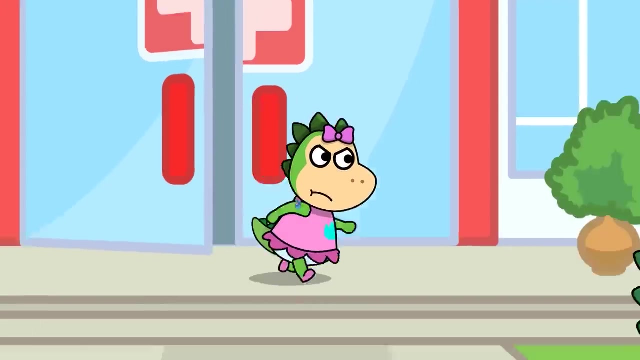 It's like a mosquito bite. Okay, kids, now wait outside. Sparkle will join you in a minute. Take a seat, Sparkle, Hmm, Sparkle, Sparkle, Sparkle, Sparkle, Sparkle, Sparkle, are you done? 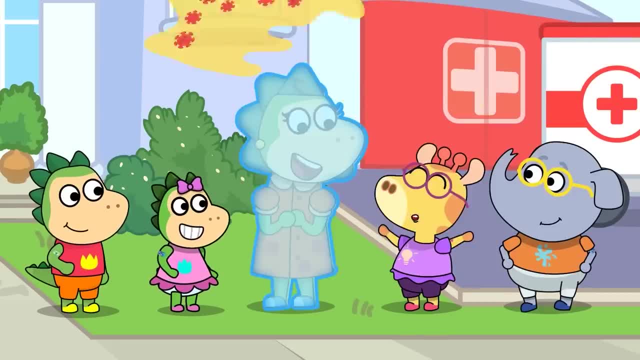 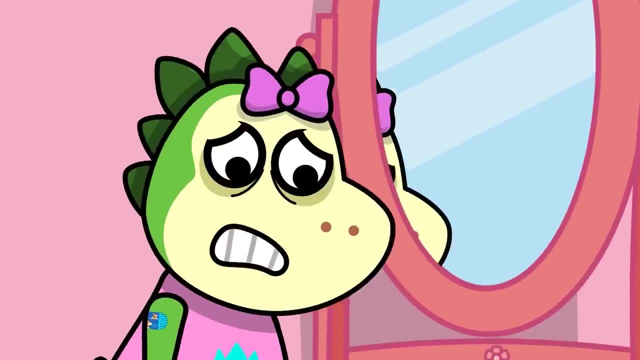 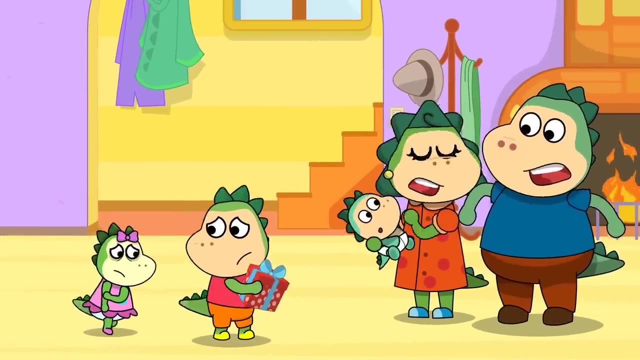 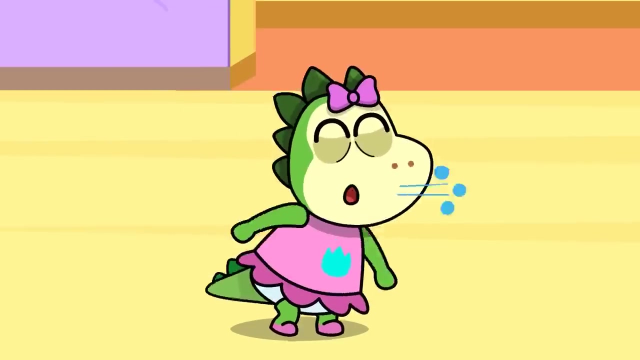 You are so brave. Great job, You did it. I don't feel so good. Sparkle, are you ready Ready Sparkle, you don't look so well. No, Sparkle, I'm fine, Achoo. 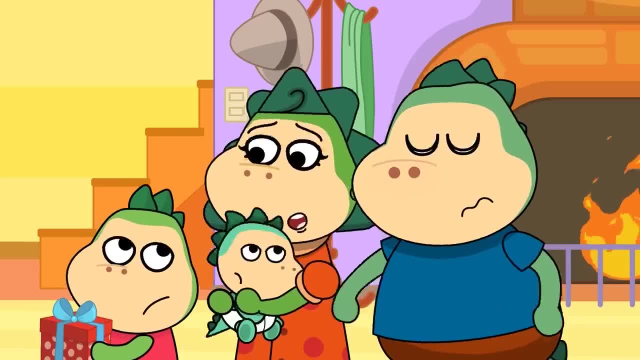 Achoo, I don't think you can go to Poem's birthday party. Sparkle, where's your band-aid? Huh, I faked it, I didn't get the shot And now I'm sick. It's not fair. 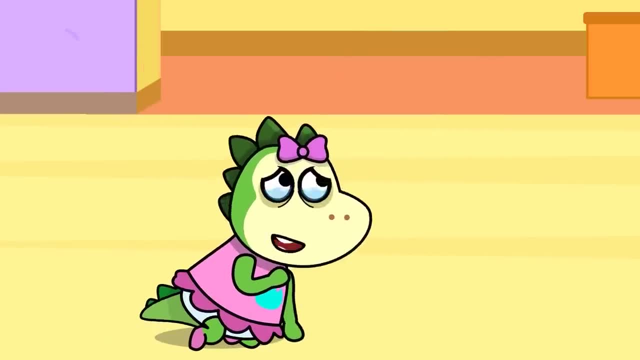 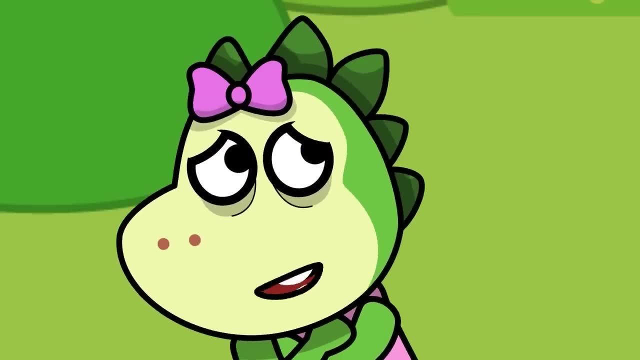 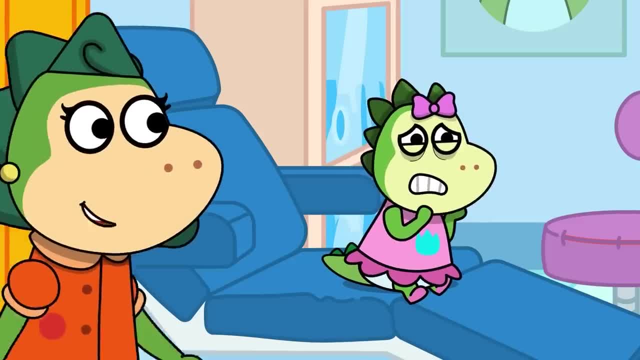 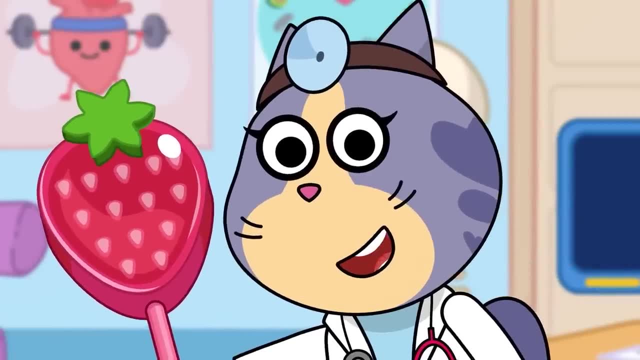 Sparkle, Sparkle, Sparkle. Close your eyes. We're excited, It'll be quick. Oooh, Oh Hey, all UPON THE NEWS, WHAT WILL WE BE DOING? That's it. Uh huh, Don't you dare question my ideas. 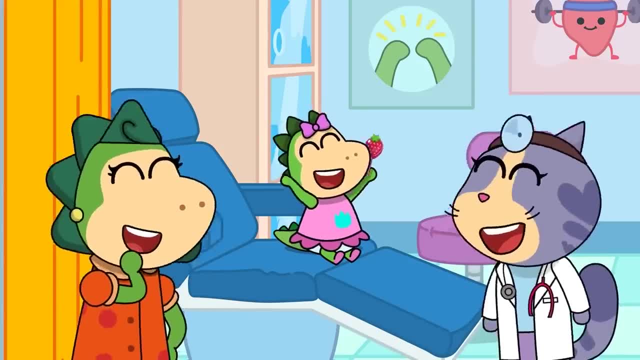 I've got a whole bunch of ideas up there. Whooo, Now let me show you all. Will you just be a'"? We're all on deck. Yes, Yeah, a big one 1..2..3.. Oh, Now it's the right beat, don't worry. 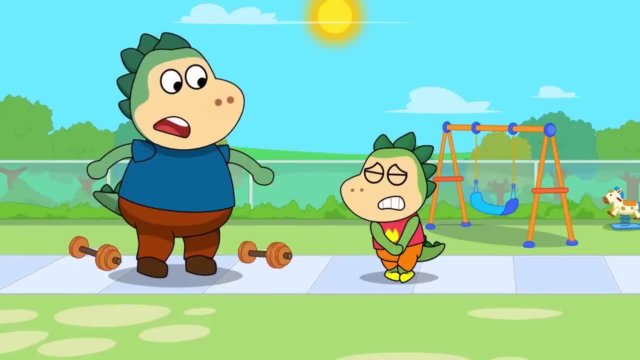 1..2..3!. 1..2..3!. Aquí vamos, Okeyy 了. Firstly… First Into the opened: cả् stim 고로… USUALLY assumed profesional was powerful And the last two were space. 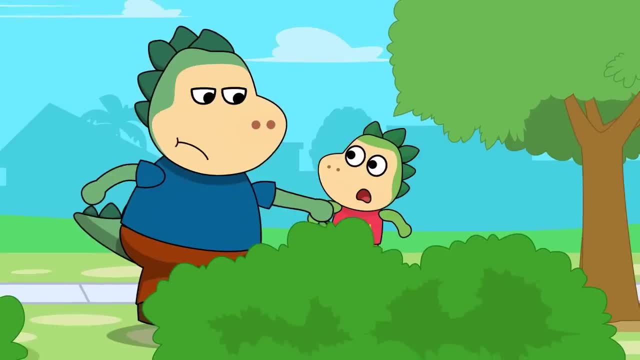 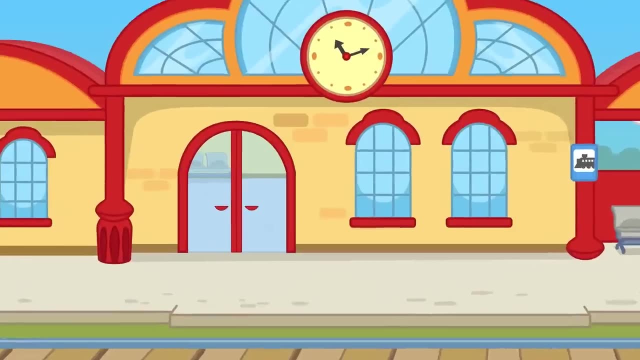 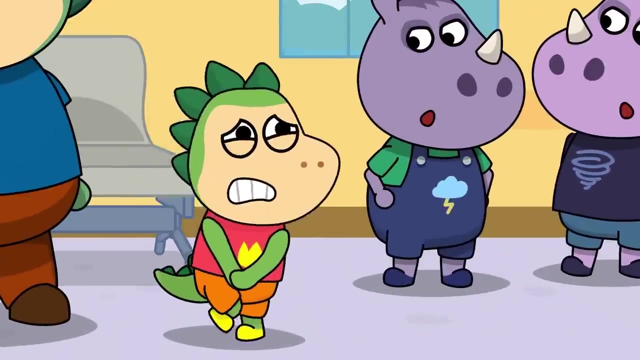 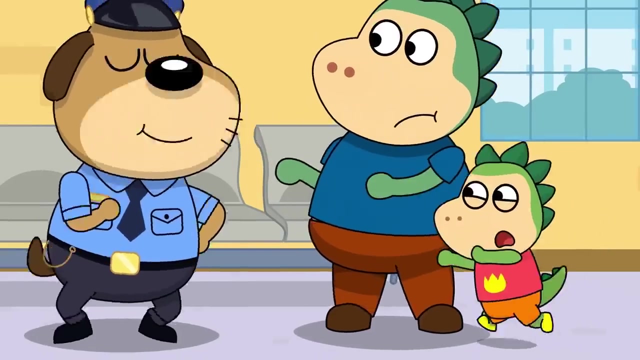 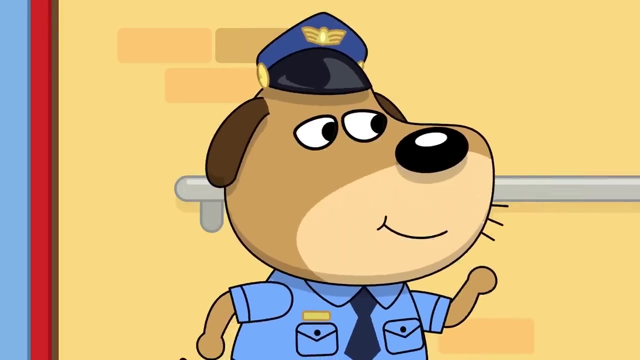 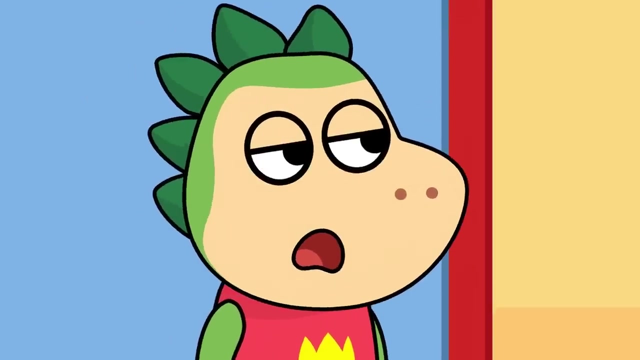 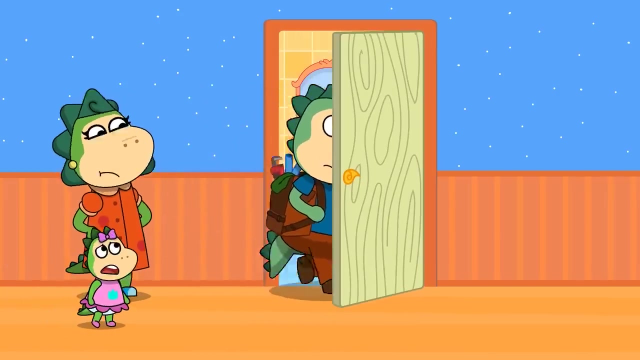 Uh-uh-uh, Hmm, Huh, Let's go. Huh Huh. Thank you, Mr Wolf, You saved us, That's okay. Emergency case: Honey, quick, I need your help. Oh, the toilet is broken. 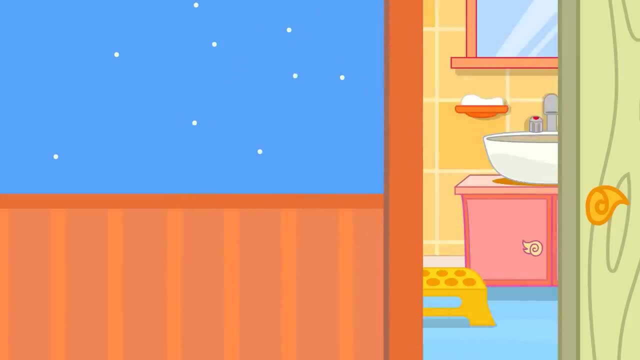 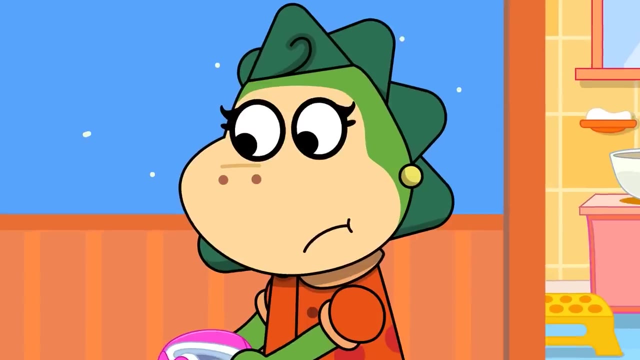 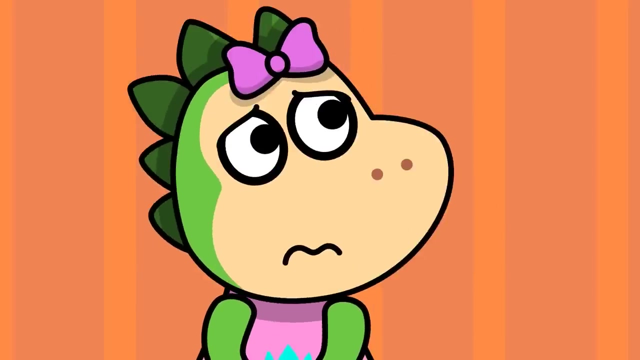 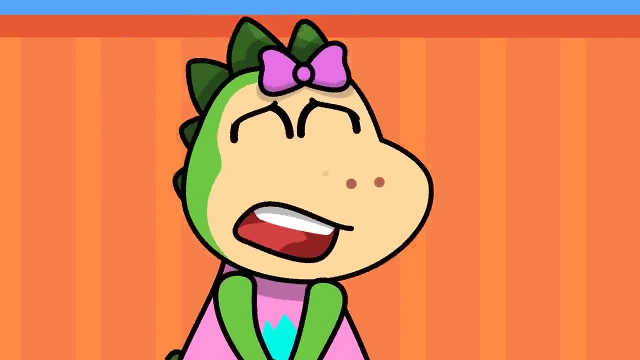 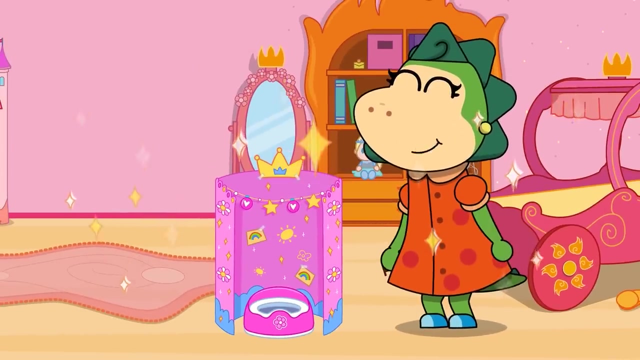 Daddy's fixing it, But you can use this. Huh, No, That's for babies. Huh, Can you hold for two more minutes? I've got an idea Almost done. Huh, Oh, Ooh. Welcome Your Royal Highness. 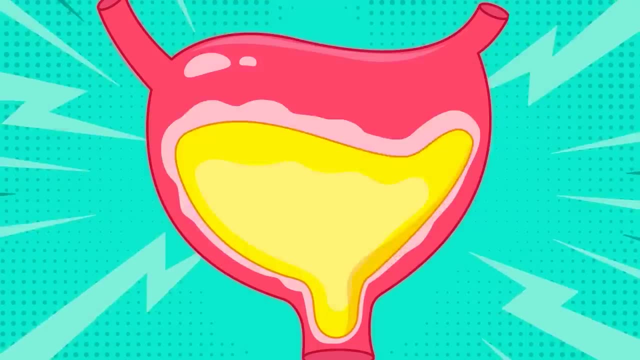 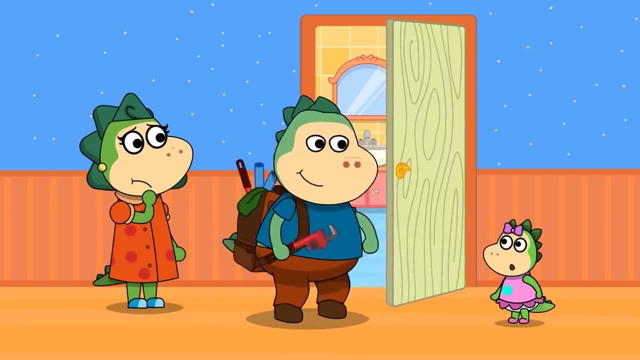 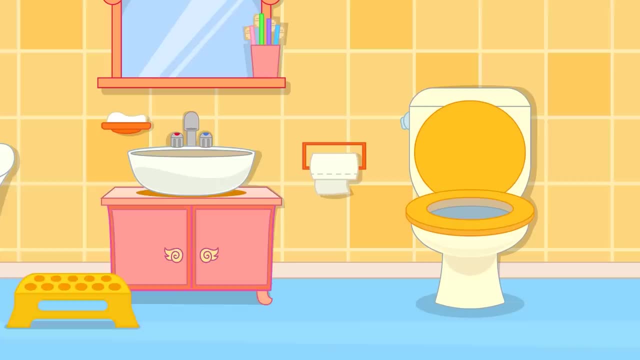 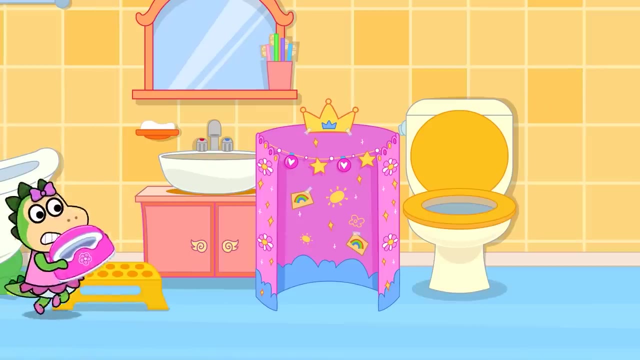 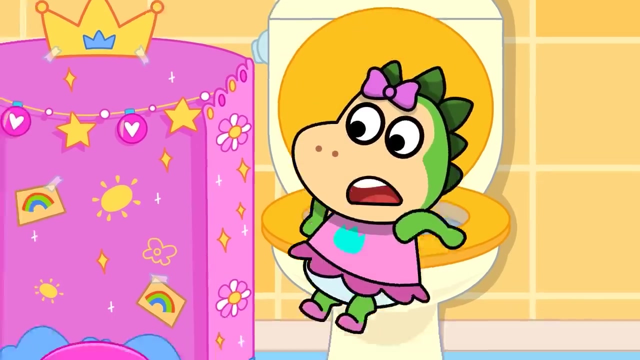 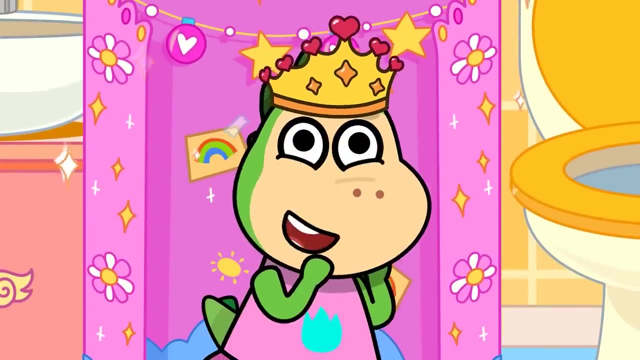 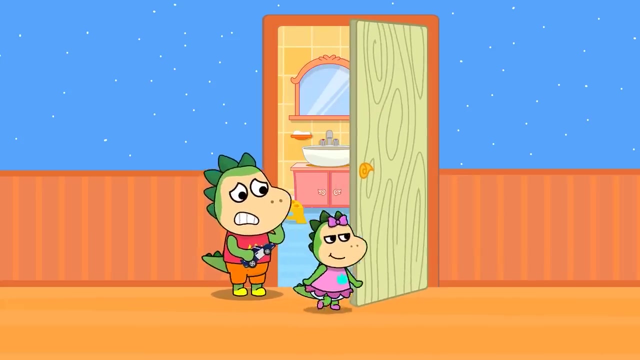 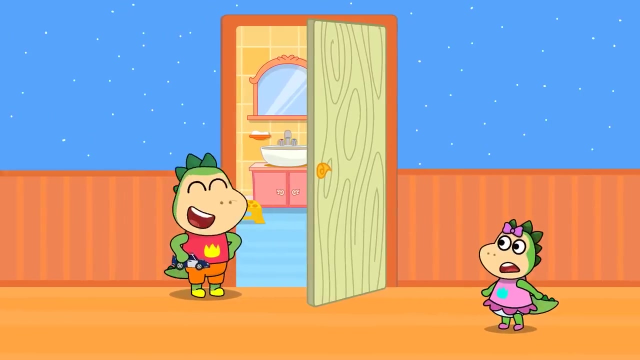 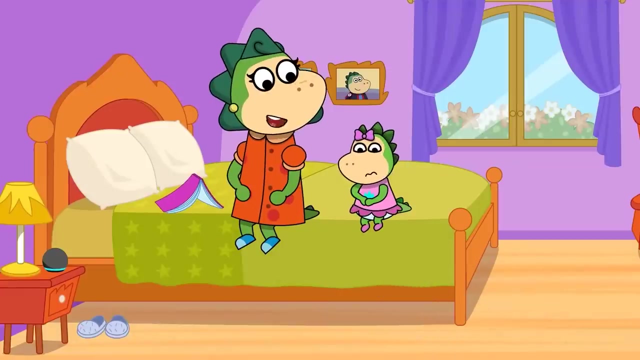 Ah, Hmm, Yeah, yeah, yeah, Which one is better? Hmm, Oh, Hmm, Ah, Huh, Perfect, Whose silly toilet. is that A baby? It's my emergency princess toilet. Huh, Oh, what is it? 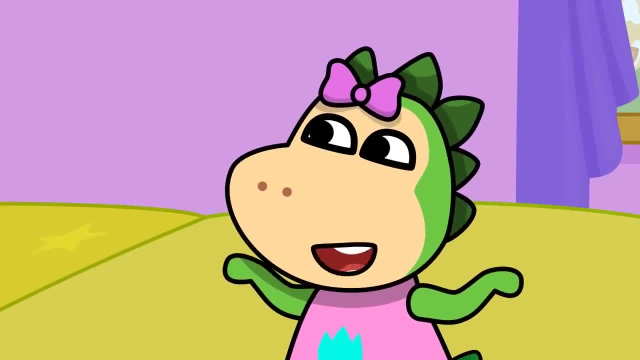 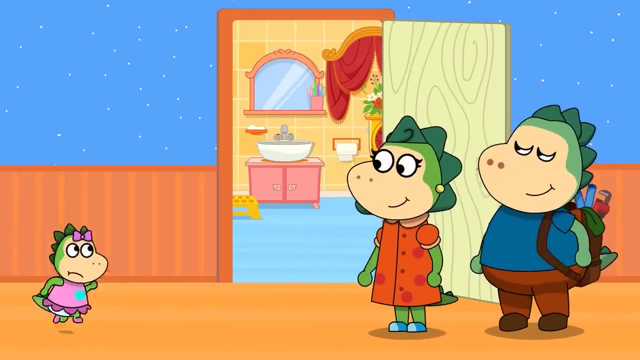 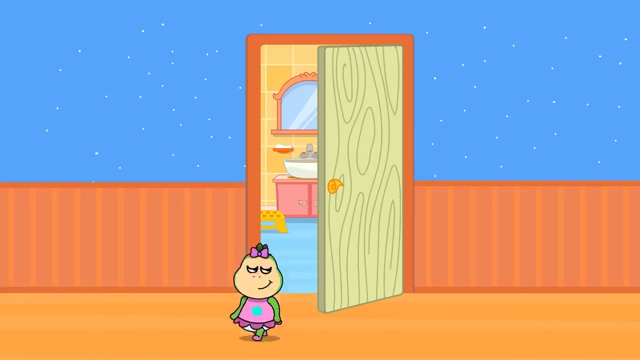 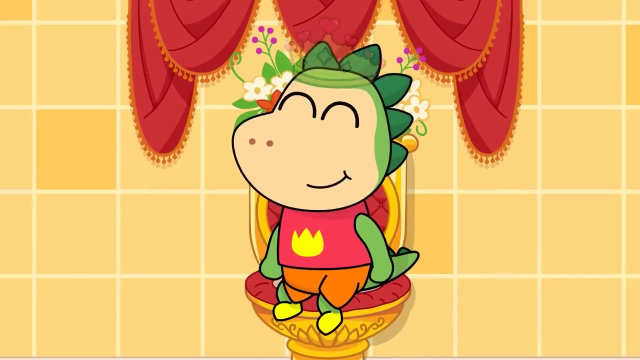 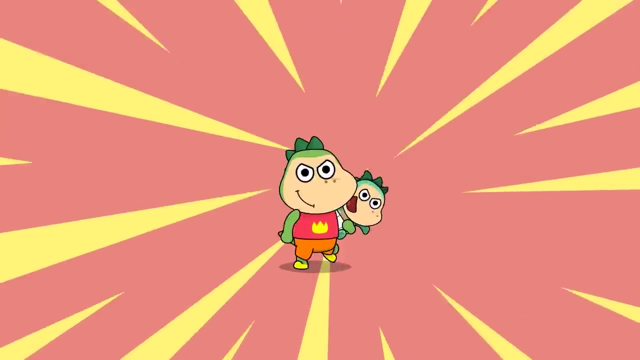 Mom, why do I need to use a baby potty if I want to feel like a princess? I think I know what we can do. Sparkle, Wow, I guess you like my funny toilet for babies. huh, Ah, They're winning the race. 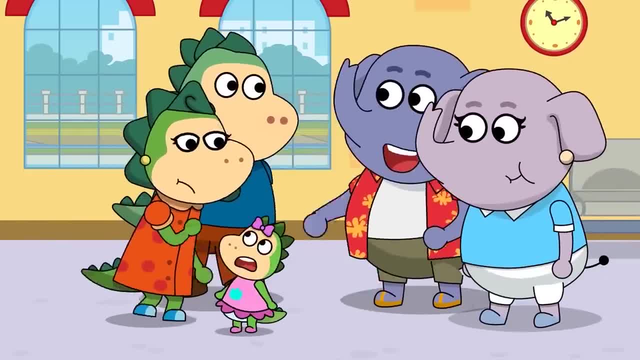 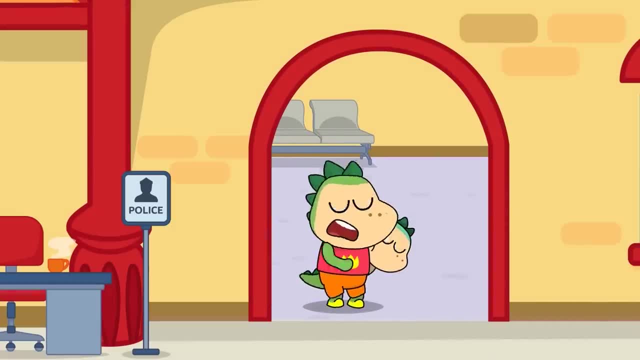 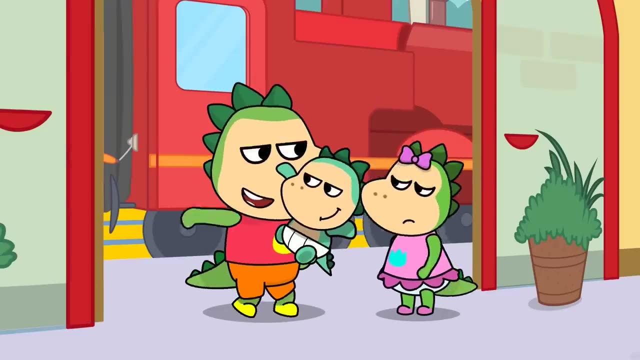 Hold tight, Goo Huh Oh, Sparkle Huh. Be careful And don't leave the station. Okay, Mommy? Ah Oh, Mommy said not to leave the station. This is technically still the station, right? 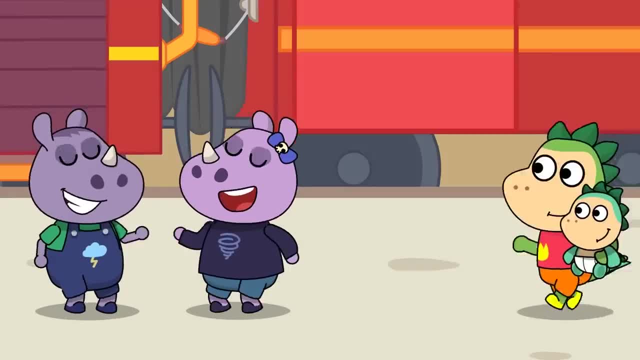 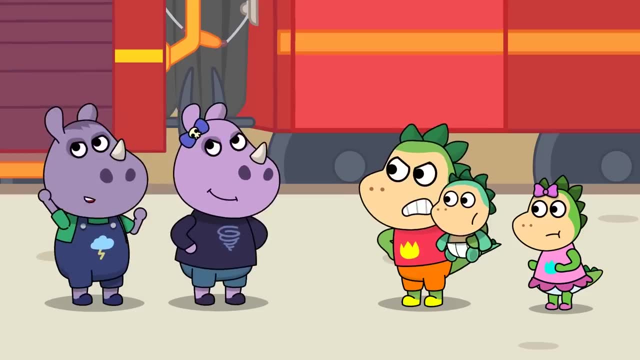 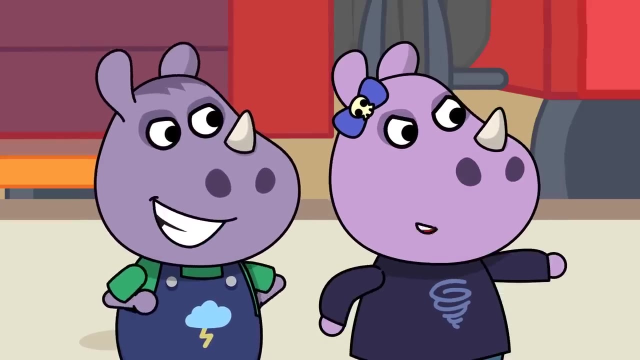 Spike. Oh, Let's have another race. Ah, Ah, Come on, let's play another game inside the train. But we can't go inside the train. Oh, Are you scared? You two are chickens. Who are you calling a chicken? 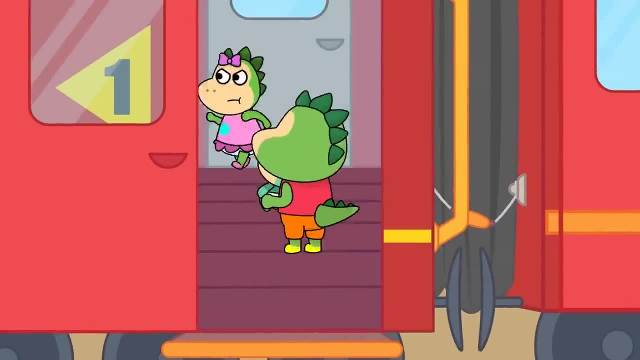 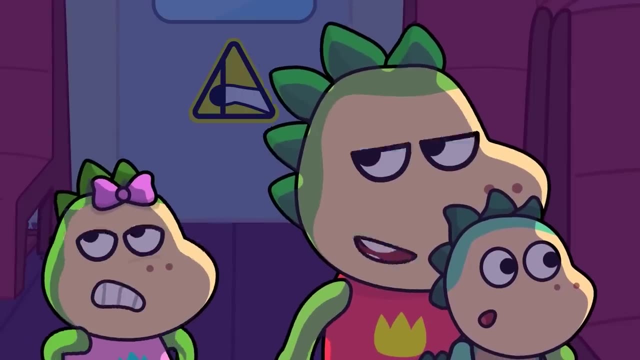 Come on Sparkle, Come on Spike. Where are they? Ah, It's them, Let's find them. Wait for us here, Goo, They should be hiding somewhere in here. Huh, There they are, Huh. 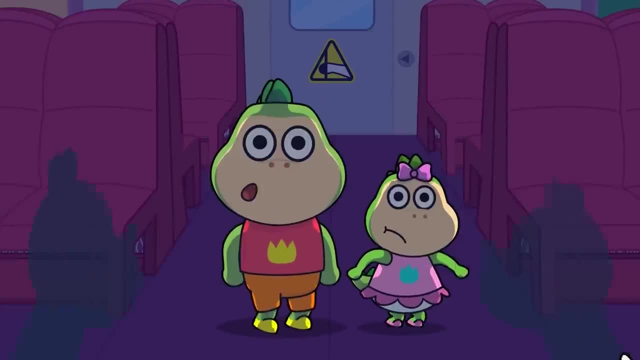 Hey, Wait a second. Ah-ha, We got you Thunder Storm. Huh, Where are you? Oh, Hmm, Let's go back, Right? Goo Ah, Goo Ah. I have to go back. 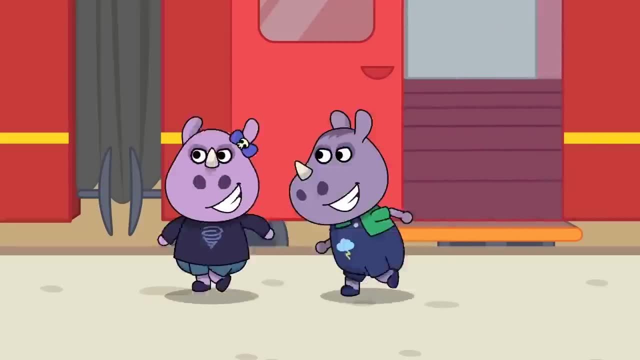 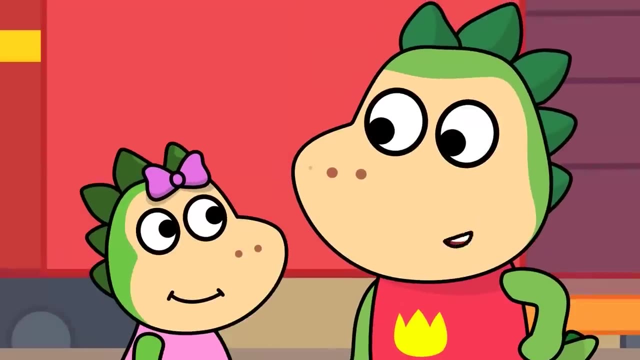 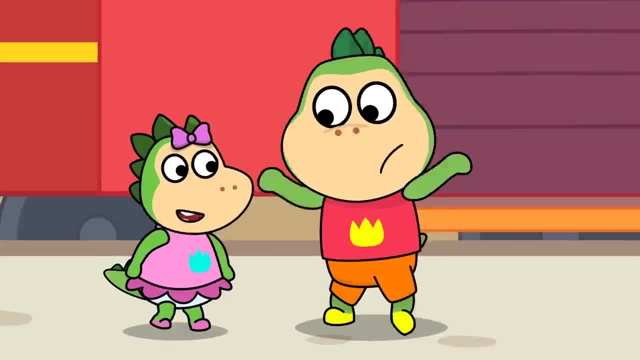 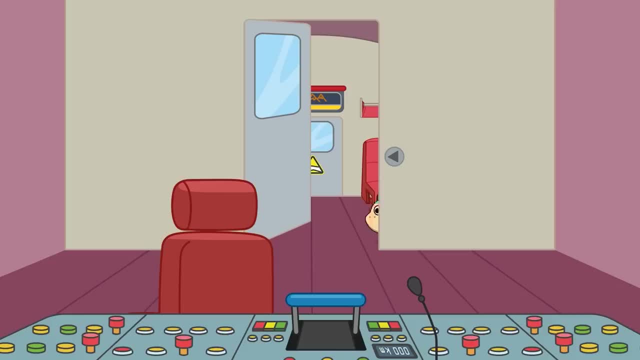 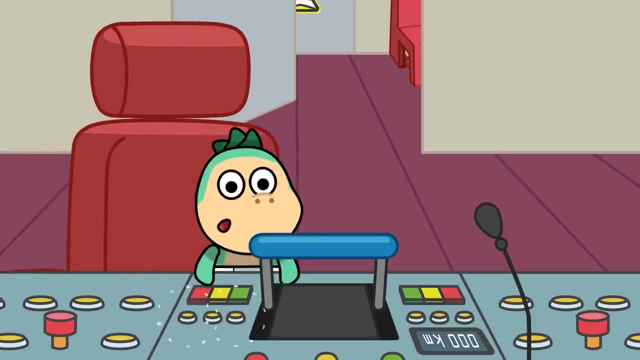 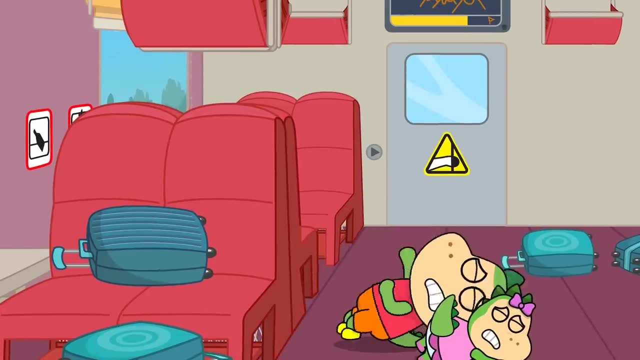 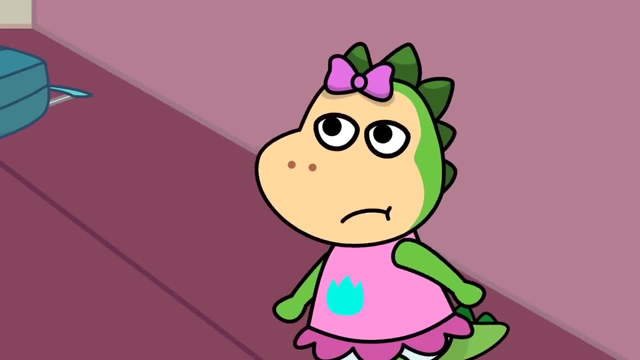 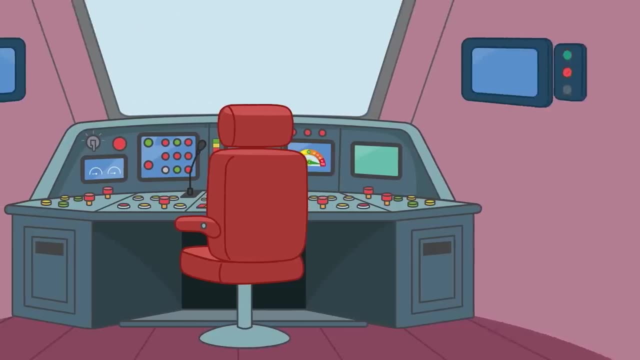 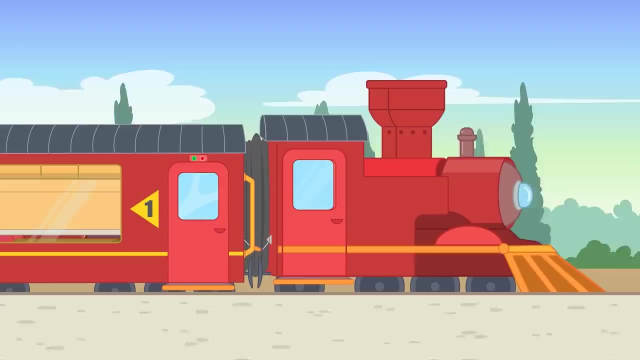 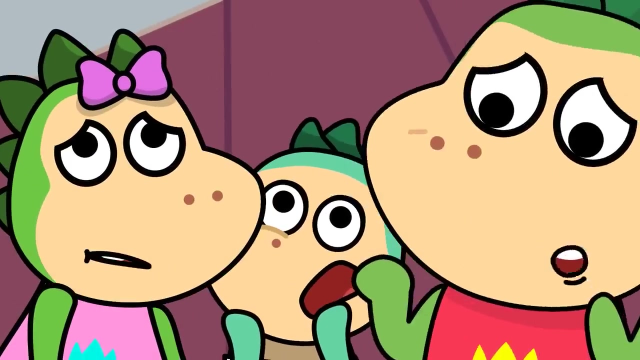 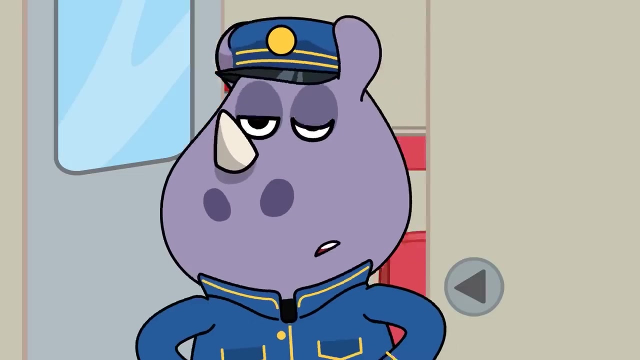 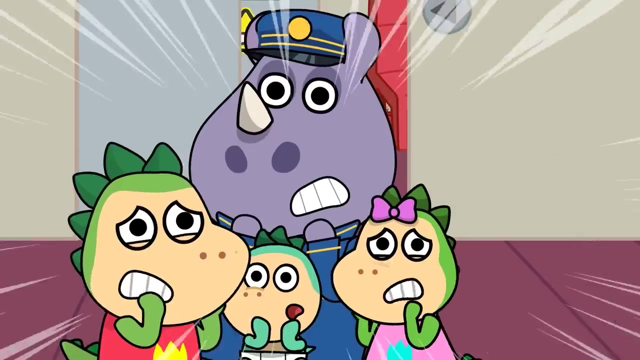 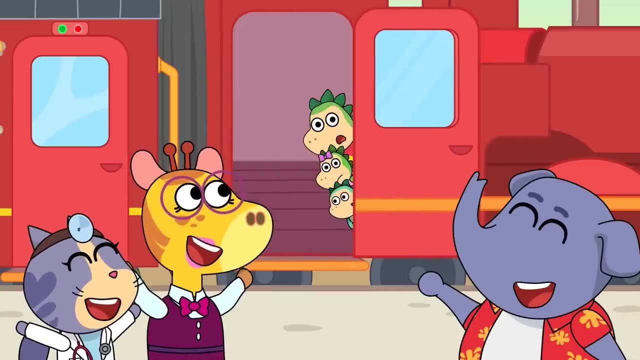 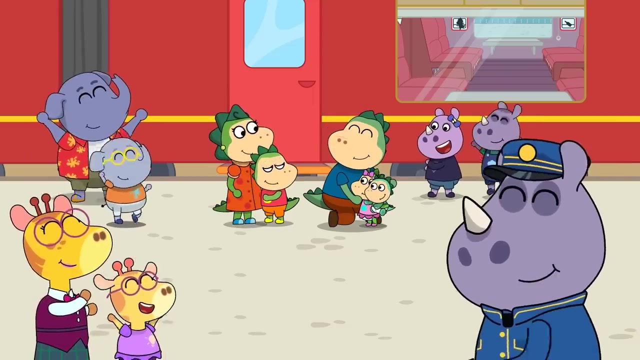 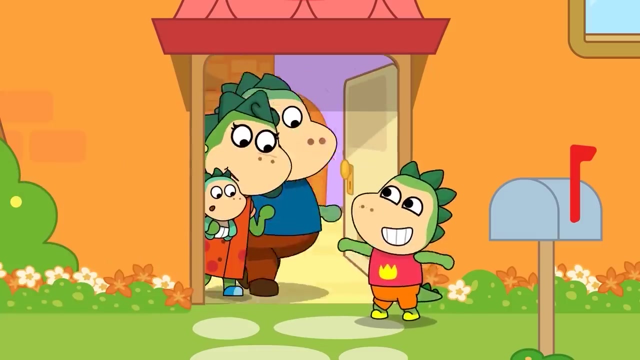 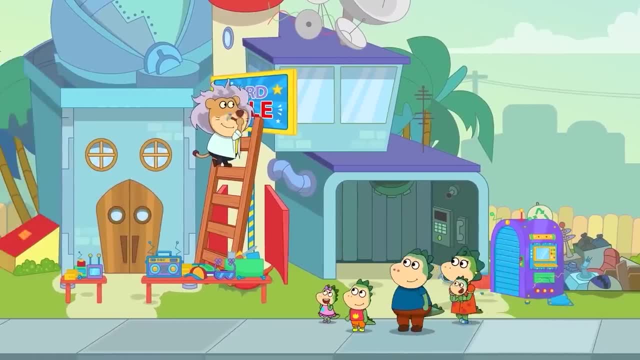 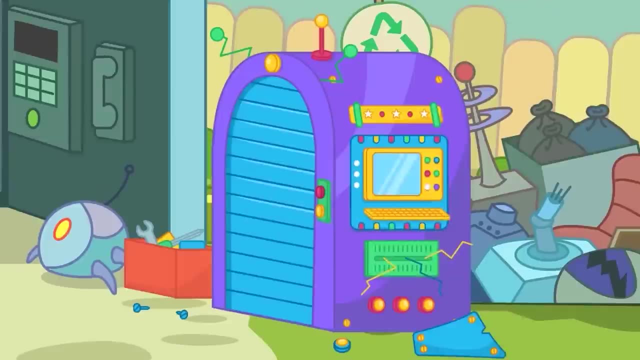 Professor Roar is having a yard sale. So Professor Roar is everything for sale. So Professor Roar is everything for sale. Welcome, Yes, everything but the collar booth. Welcome, Yes, everything but the collar booth. 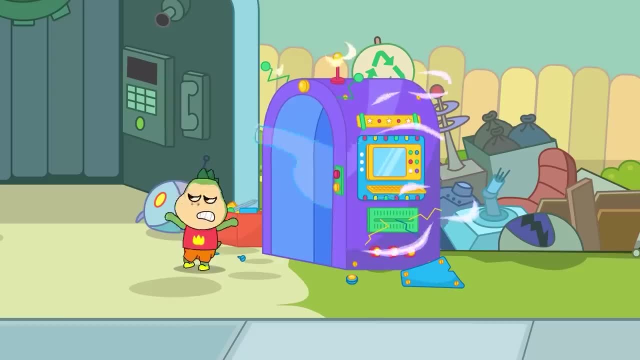 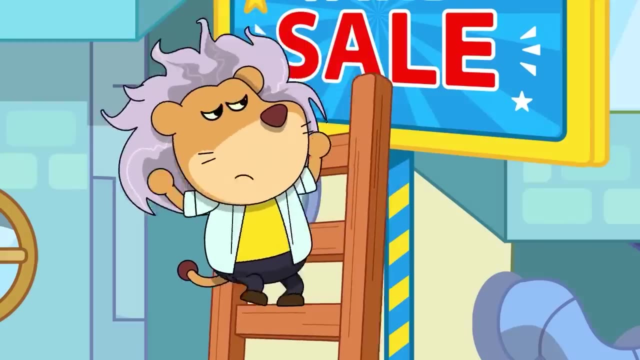 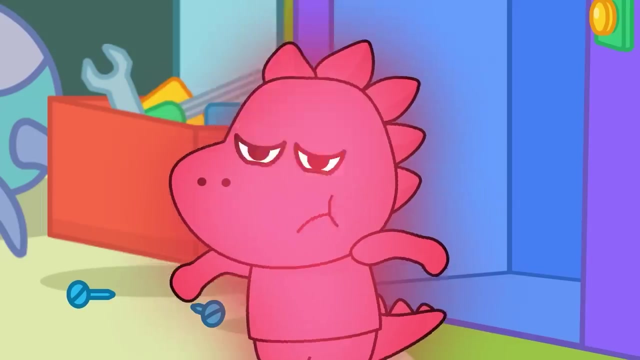 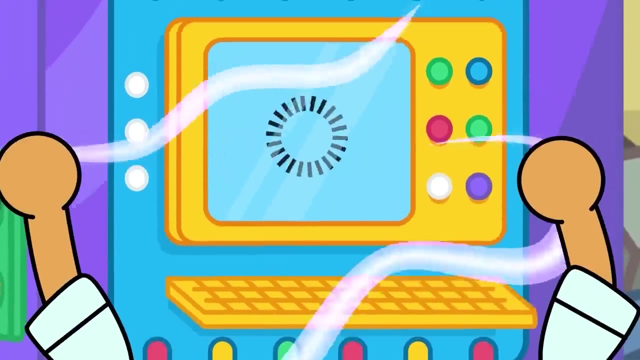 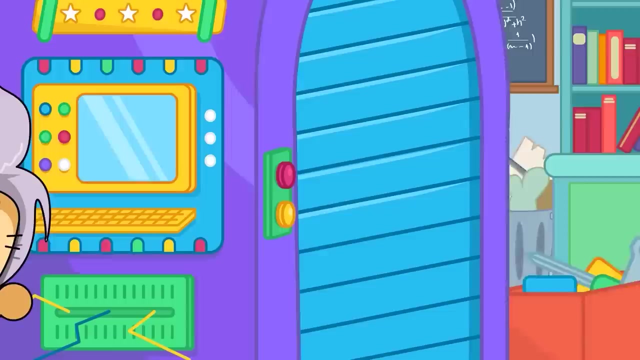 Spike, you heard, Professor Roar, It's not for sale. No, Don't go in there. What happened? Let me fix it. Oh no, It's broken. What are we gonna do now? This should do it. This should do it. 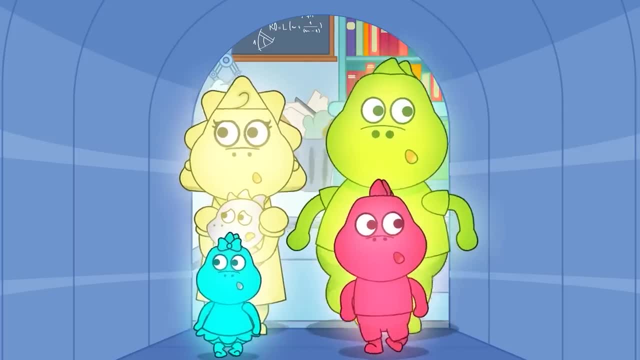 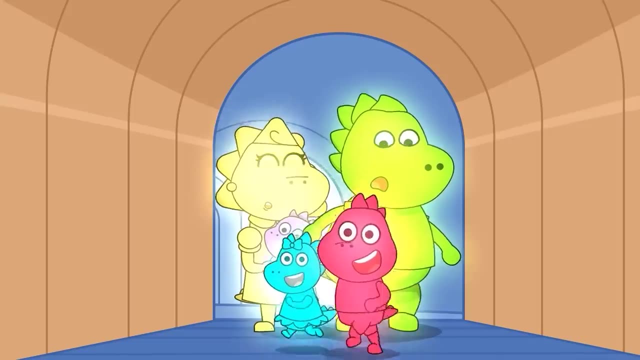 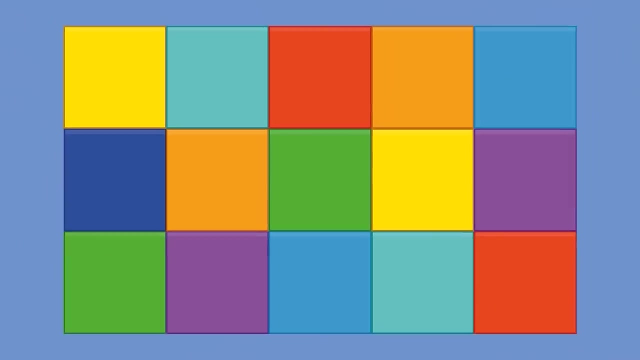 All systems connected. This will change you back to normal. Are you here, Professor Roar? You won't believe what just happened. You won't believe what just happened. Pair the squares by colour to find the exit. Pair the squares by colour to find the exit.